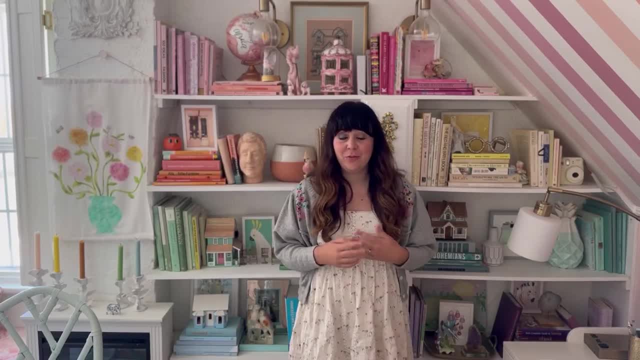 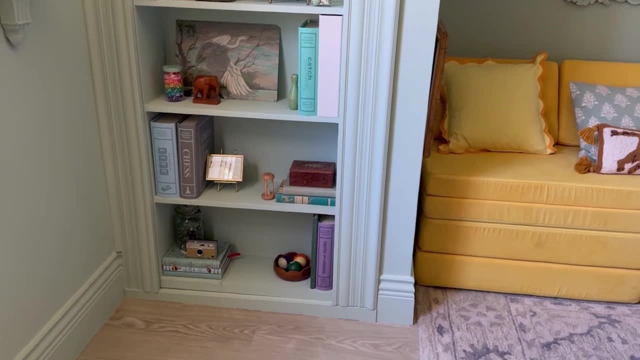 Hello, I have a really great project for you today. Okay, so a few weeks ago we took a boarding door in my playroom and we made it shelves and the whole point was to put games on them. So I don't know if you noticed, but I put some just like white empty book boxes on them. 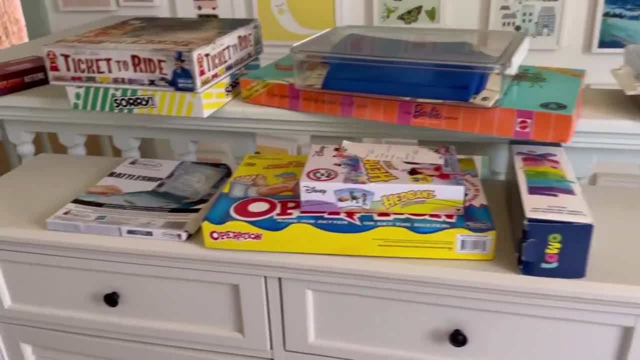 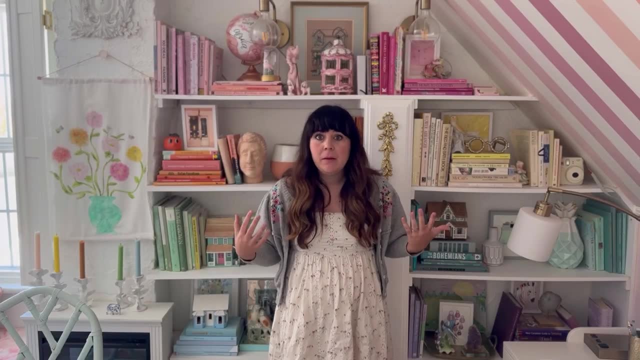 and that is because board games come in the ugliest boxes and they're not uniform and it makes me nuts. I just want them to be beautiful and to be able to be seen, and so we play with them more. So I want the beauty to match the function. So I do own a good amount of pretty. 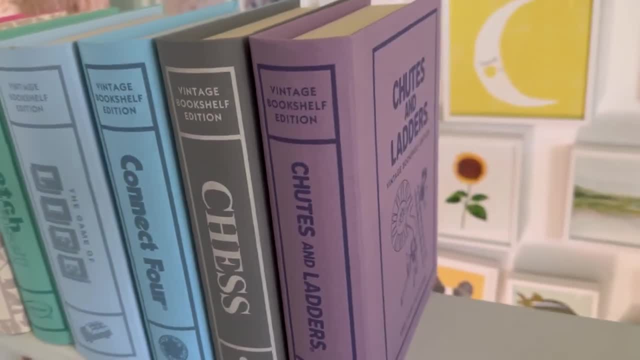 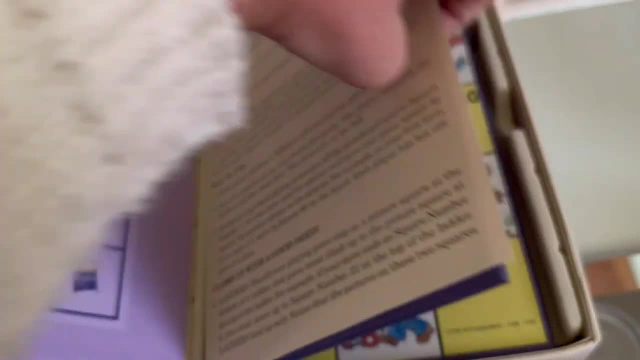 games, and this is also where my inspiration came from. They're called bookshelf vintage edition games and they're expensive. They're like 40 to 45 dollars a piece and they only come in a limited amount. So I've bought all the ones I want. Well, I mean, never say never, but I would like more. But 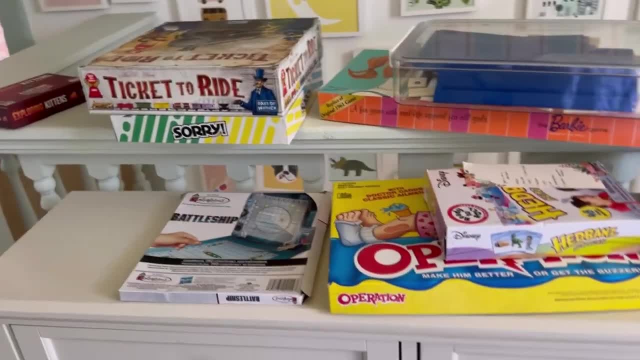 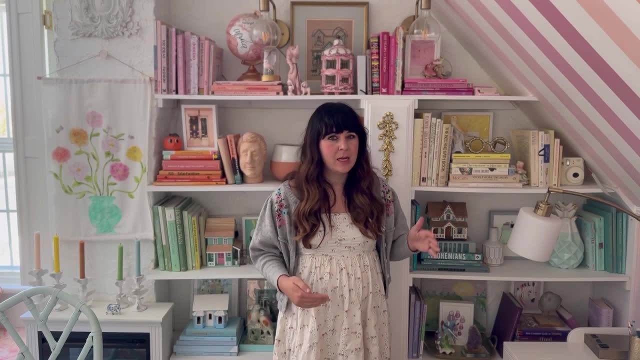 also, I just already own some board games that I would like to put in these book boxes. So the first thing I did was, before I even ordered the book boxes, I opened the games and I kind of saw, like what size these could go in, and then 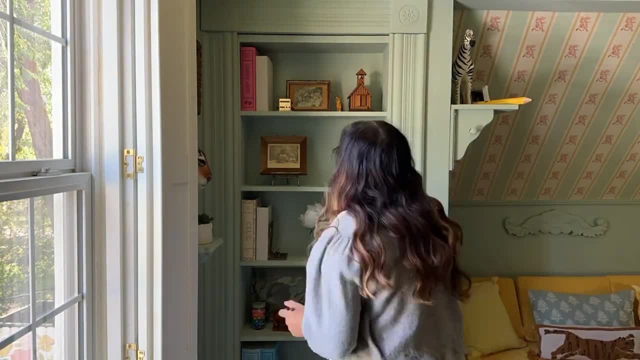 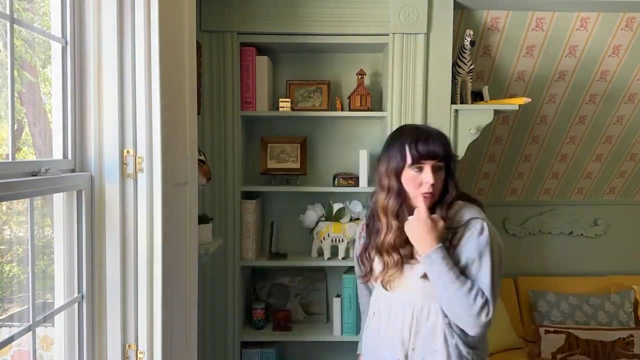 now that the boxes are here, I'm actually putting the board games in them to like make sure they do fit, and so that's like the big first step. And each of my shelves is going to have a different color, Like I'm going to do it kind of rainbow-ized, so I need to know which shelf I want each book on. 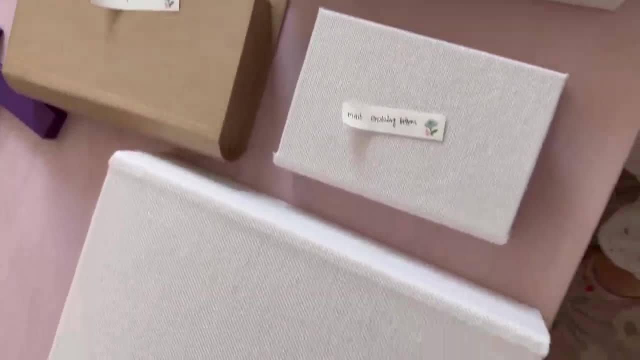 so I can know what label to put in what color on each book. For all of my books. I ordered these plain white linen books For these. I ordered these plain white linen books. I ordered these plain white linen books For all of my books. I ordered these plain white linen books For all of my books. I ordered 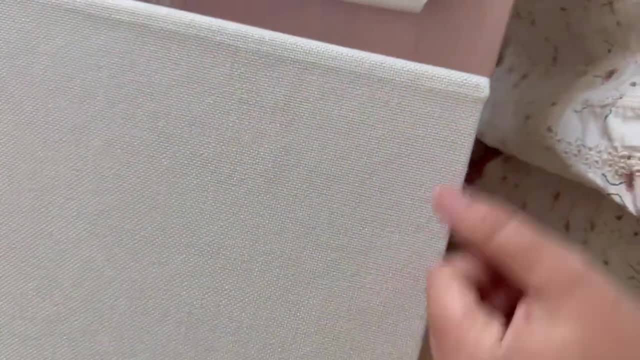 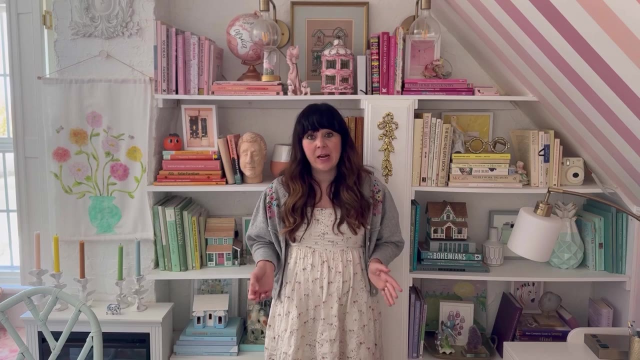 book boxes and the quality is great. There's like a little magnet on the inside. but the white is so boring to me and I don't like it, So I'm going to experiment with dyeing them, and I was really worried about this because I didn't want to ruin the book boxes. but what ended up working for me? 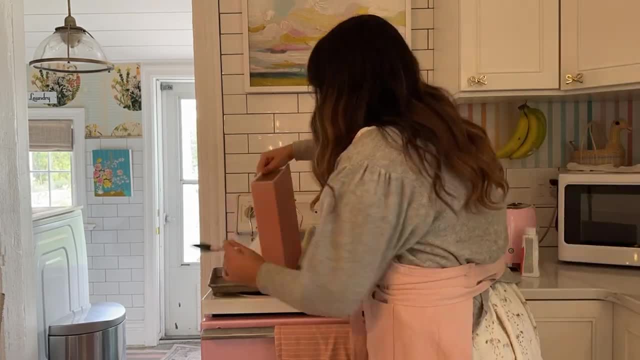 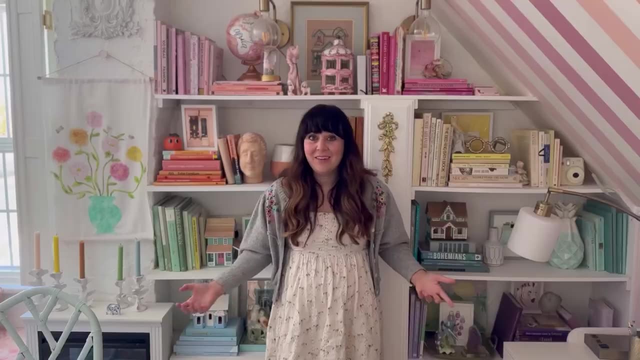 is, I boiled some water, I put about a tablespoon of dye in it and then I used a paintbrush to paint on the dye and I didn't ruin it and it worked really good. My other option I was thinking about was watering down some paint or using some fabric paint, but this worked so well I didn't need to. 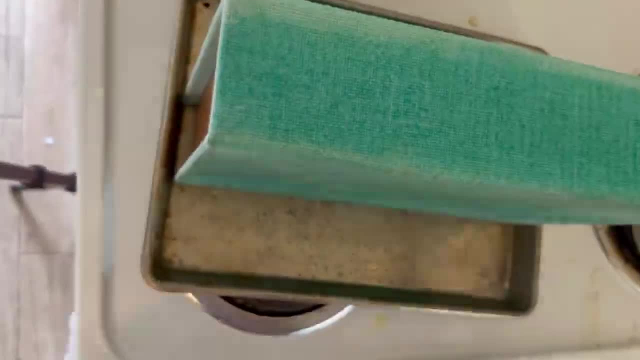 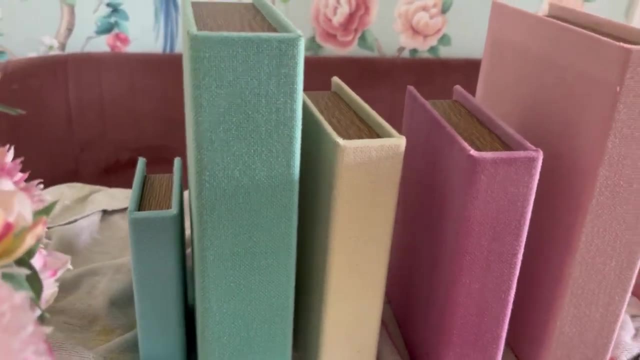 I made sure to have a cookie sheet underneath while I was doing it to catch the extra dye. and then I had a thick towel on my table and that also caught dye and I'm glad I didn't dye my table because there was a lot of dye. So make sure you're. if you do this, it's nice and thick that towel, or 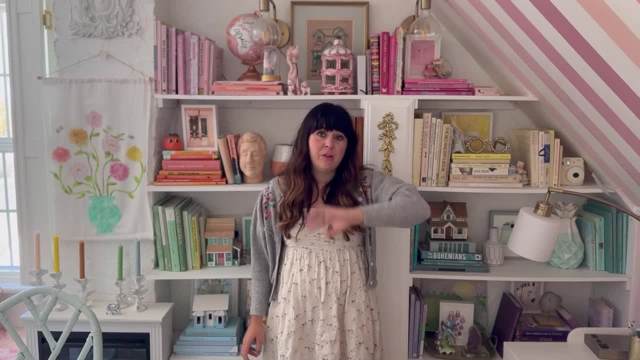 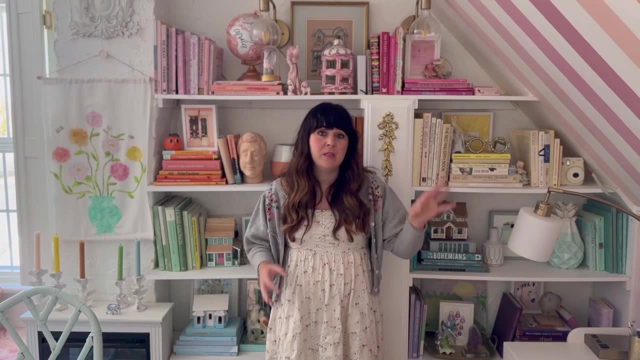 you do two towels. One thing I do wish I had done is flip over the books while they were drying, because some ended up kind of ombre, which looks cool. but I think if I would have flipped them back before A few times the dye would have all like rushed out. So I kind of want my books to look like. 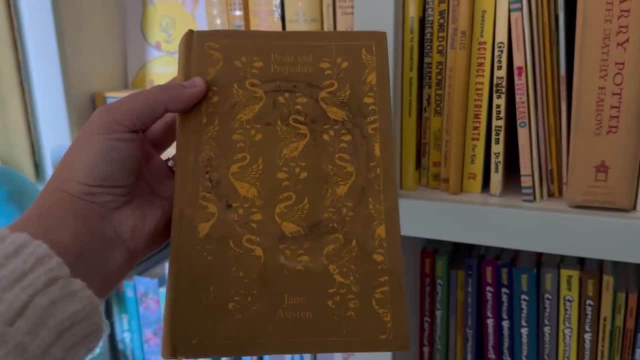 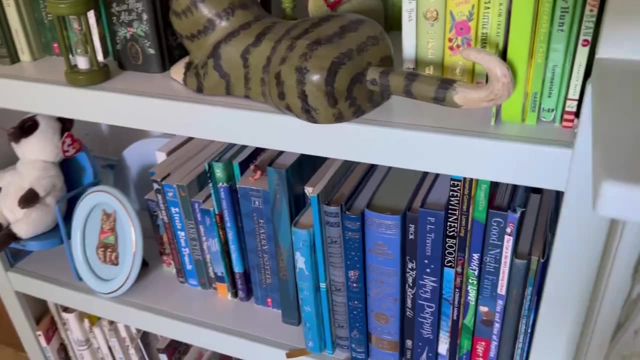 penguin cloth bound books. I don't know if you've seen them. I have a few. They're actually in a bit of rough shape, the ones I have, but what they have is a rectangle border. They have the name of the book and the author in simple font, so I'll just do the name of the game, and then they also. 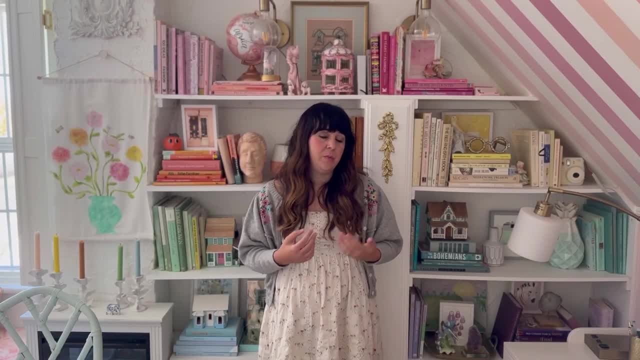 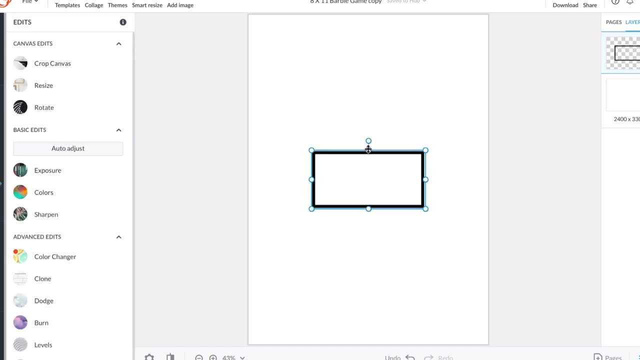 have like a motif that speaks to the book, and so I'll do something that speaks to the game. So I am designing all of mine. on the online software PicMonkey, I'm going to pay a little bit to use it, but I'm used to using it, So that's what I'm doing. 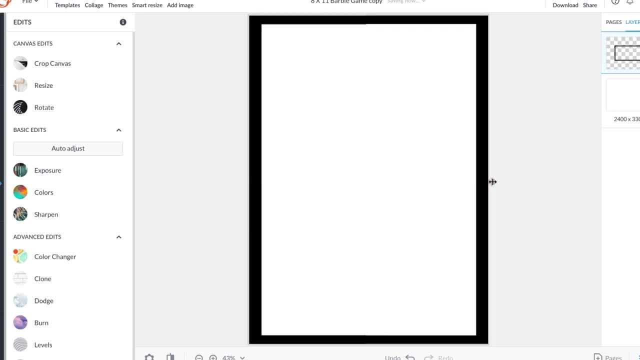 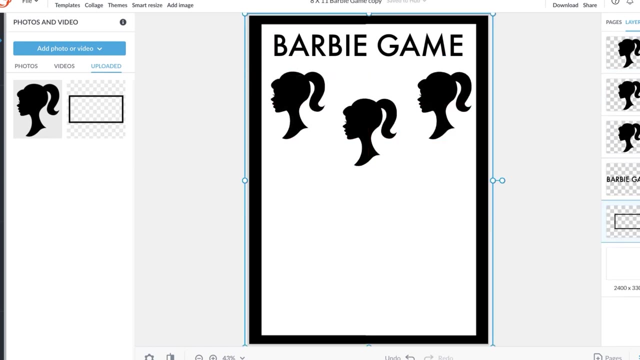 I'm making the border and then I'm adding the name and adding the motif, and it took me probably an hour to make the first one. I was like, oh crap, I have seven games I need to do. but once the first one was all figured out, I was able to easily like just tweak the first design and switch it out for other. 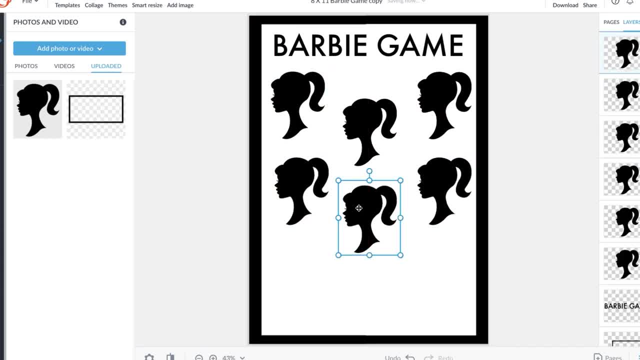 things that worked, So it did take some time. I'm going to be cutting all my stuff with a Cricut, so I've saved my game. I'm going to be cutting all my stuff with a Cricut, so I'm going to be cutting all my stuff with a Cricut, so I've saved my game. 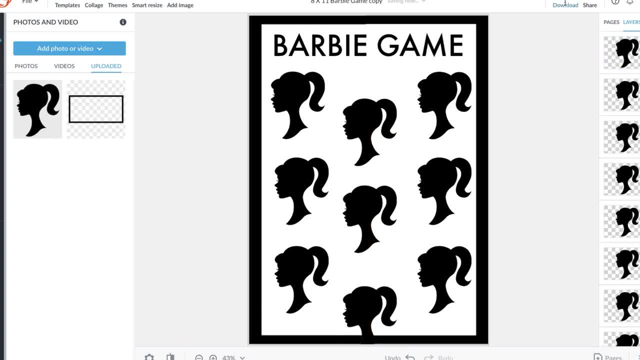 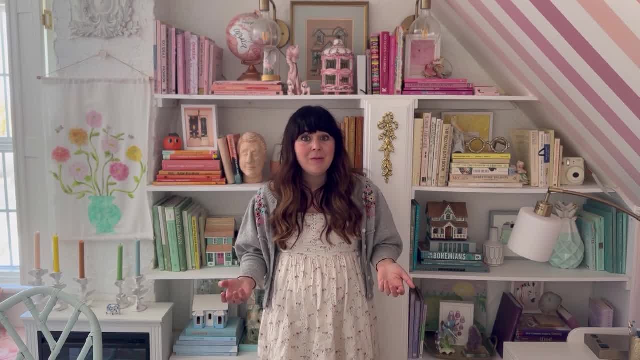 labels onto Cricut Design Space and the link to that is in my description. So if you have, if you're going to make this and you're going to use a Cricut- which is the best and probably only way to make it- then you can use my files if you would like. So now that the design is done, we need to cut the vinyl. 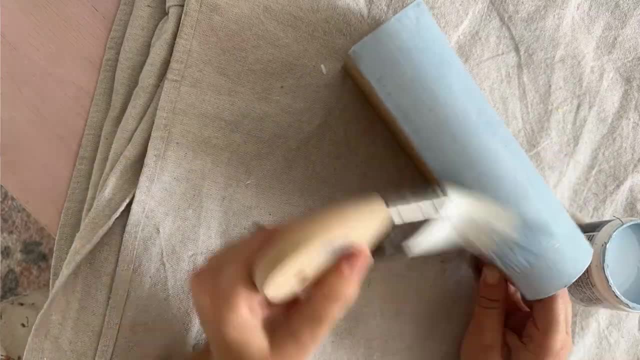 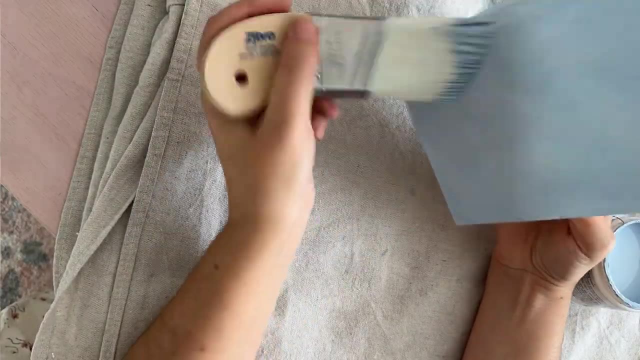 so that it can be put on the books. So I have one paper mache book that I'm going to use, and for that one, instead of dying it, we just painted it, and on that one only I'm going to use vinyl, and the rest of them I'm going to use a paper mache book. So I'm going to use a paper mache book and I'm going to 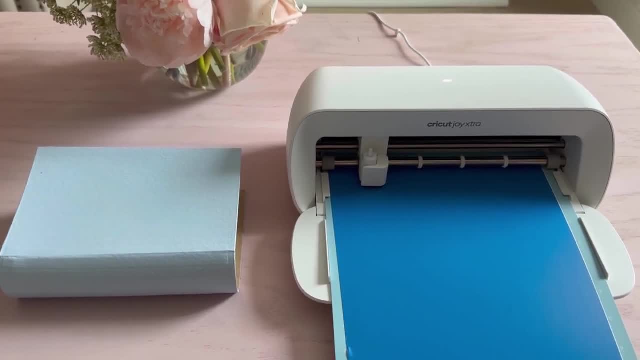 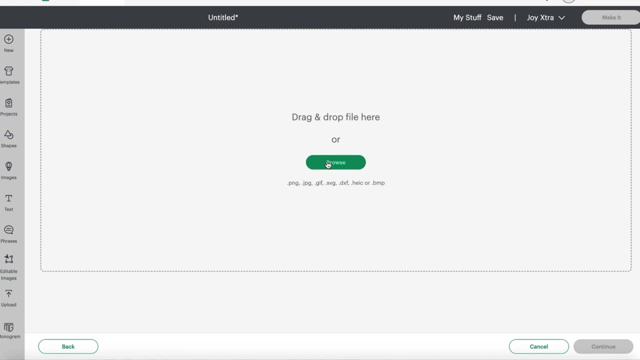 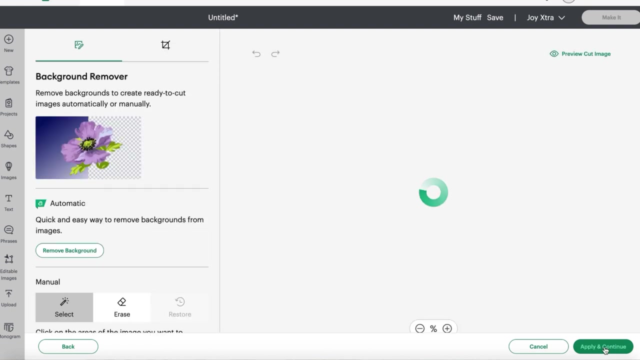 use iron-on material. The first thing you need to do is to upload your design into Cricut Design Space. So I saved mine as a PNG from PicMonkey, I upload it onto my canvas and when you're uploading it you need to decide which areas are the background. I mean, that's really easy. any of. 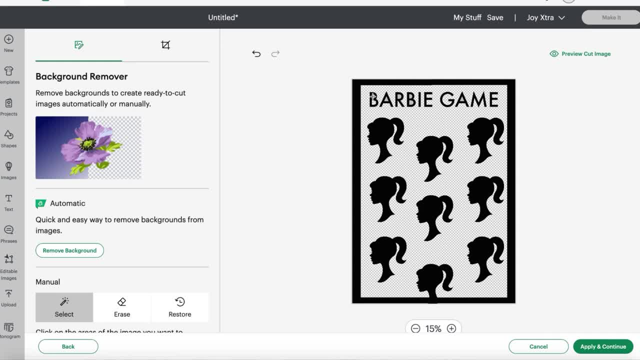 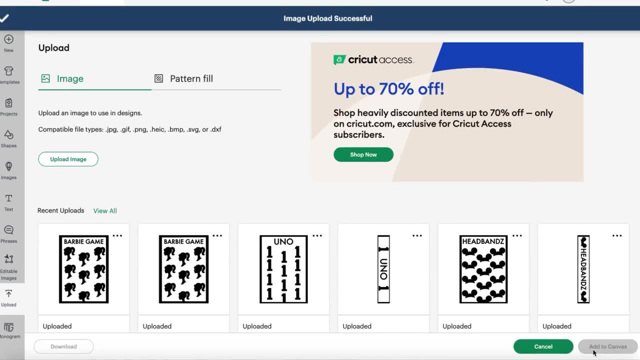 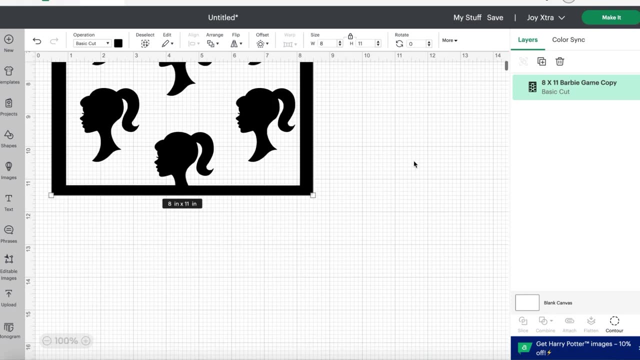 the negative space you need to click so that those don't get cut, and then you upload it as a cut image and you put it in to your Design Space canvas. It is going to come up as like a wild size, Even though I sized it correctly in PicMonkey. So then I'm just going to change the dimensions. 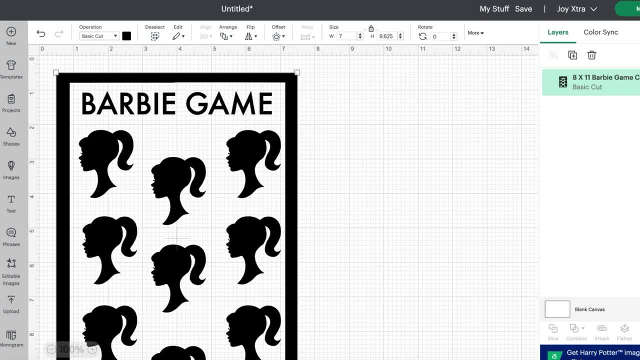 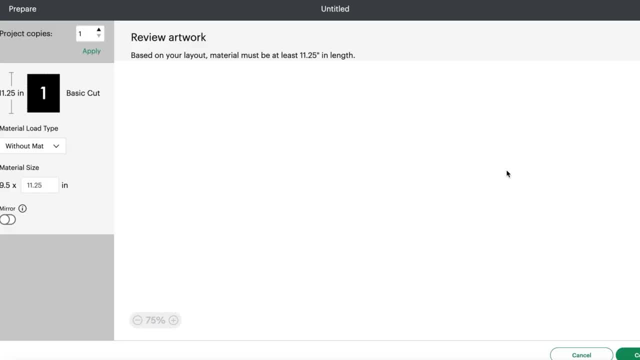 on it, so it's perfect. Once the label is in Cricut Design Space and you're happy with the size, I click on make it and then you need to decide: are you going to cut it with a mat or without a mat? So for smart materials you don't need a mat If you're using older materials and putting 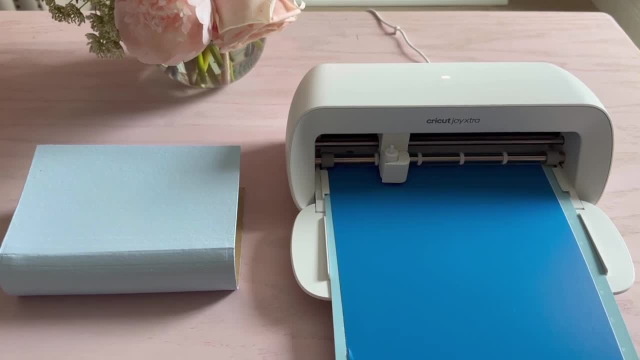 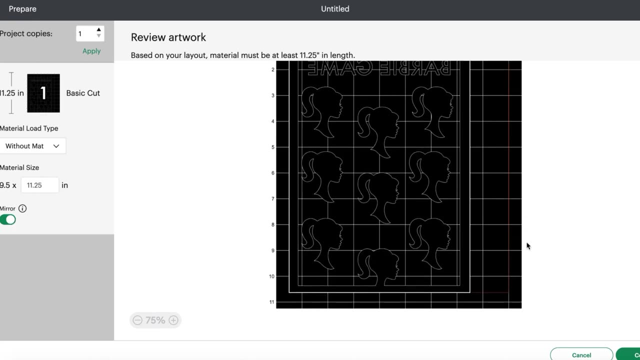 it on a mat. you click with a mat And once you confirm that, you're going to go to the next page to verify. the art looks good, And this is where, if you're doing an iron-on, you have to make sure to mirror it. So this is going to cut it backwards. so then, when you iron it on, it goes on the correct. 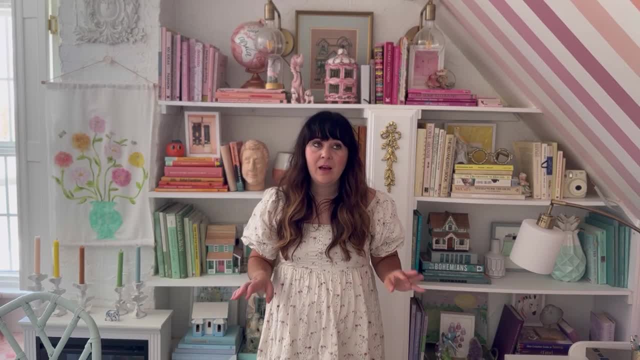 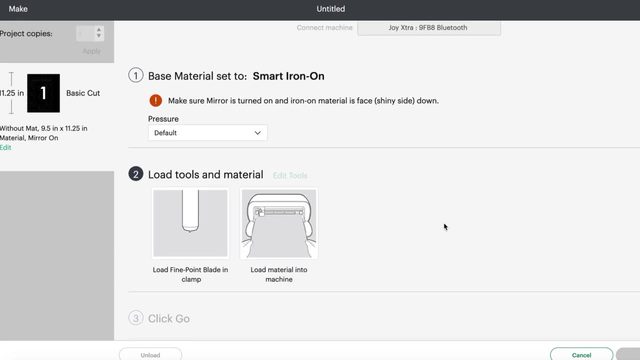 way For the normal vinyl. you don't need to mirror it. I made that mistake. And then you have to set the base material. So again, you just need to know what you're cutting and if it's not on the short list, you can click browse all materials and select, like the iron-on vinyl or whatever you're doing. 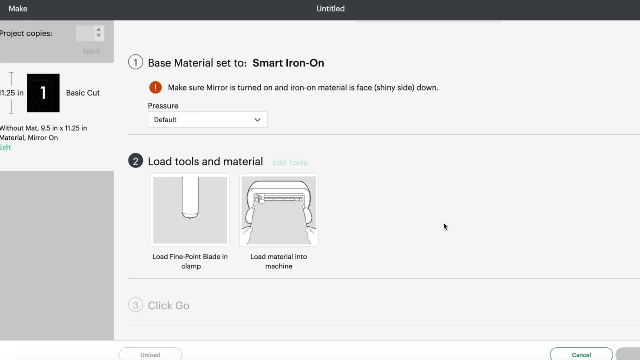 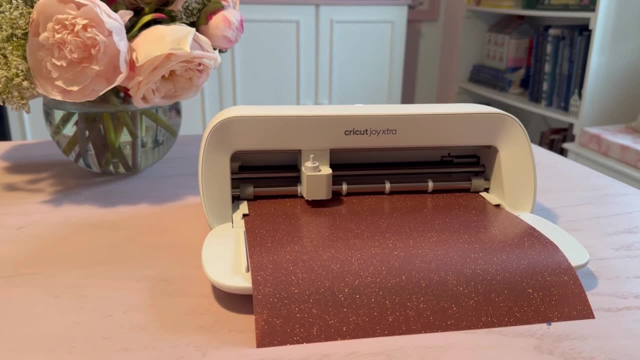 And I'm using the holographic vinyl for some and glitter for others. So you just choose the right thing, because that's how the knife knows how hard to cut down. Then all you have to do is you load your material, you push, go and the machine takes over from there and quickly cuts it. And this is. 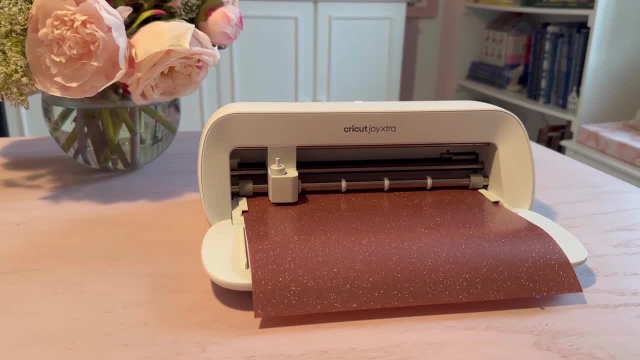 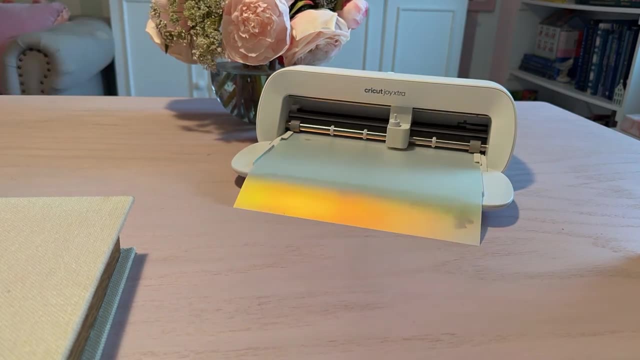 always so fun because it's like I did all the work and now it's doing what I told it to do. It's very exciting. Once it's done cutting, it'll tell you and you just need to push the unload button on your computer or your app. There's a Design Space app. I like the computer more, so it's up to you. 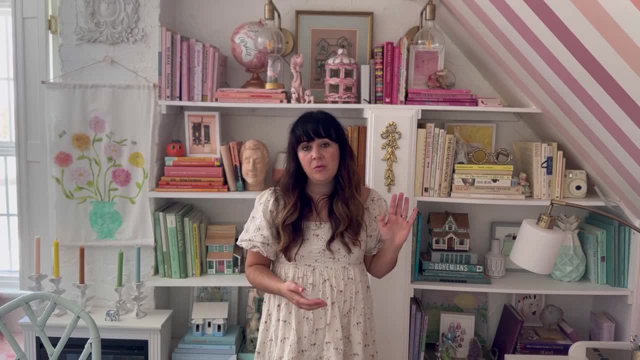 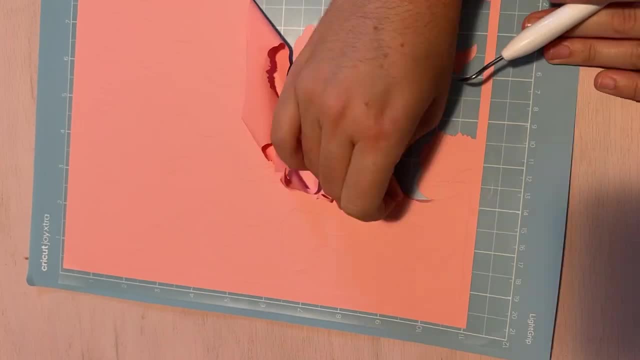 what you use. Okay, so once it's all cut, we need to put it onto the book. Before you can do that, you need to make sure to weed out all those negative space items that we selected on when we were pulling the design in. So anything that's going to be on the background, you use a little weeding. 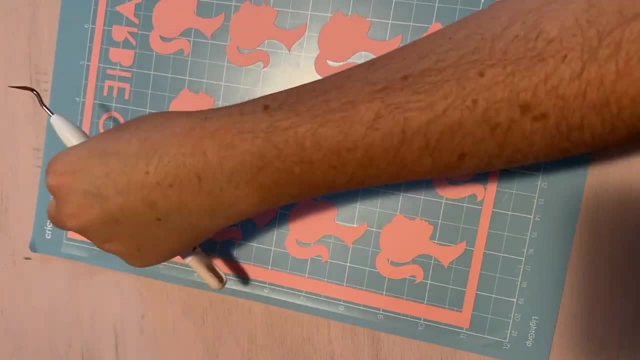 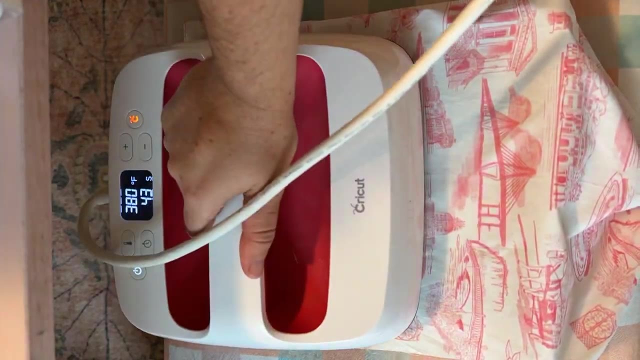 tool and you pull it out, and this is always kind of fun. It's like I don't know. it's very satisfying. So now that it's all weeded and cut down to size, you can put it on the front of the book or on the spine of the book, and it's very, very, very, very important that you get it lined up. 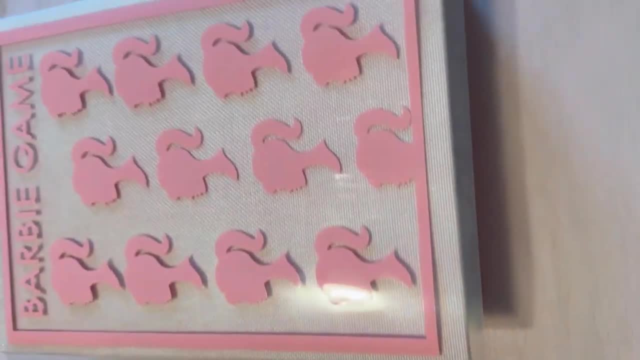 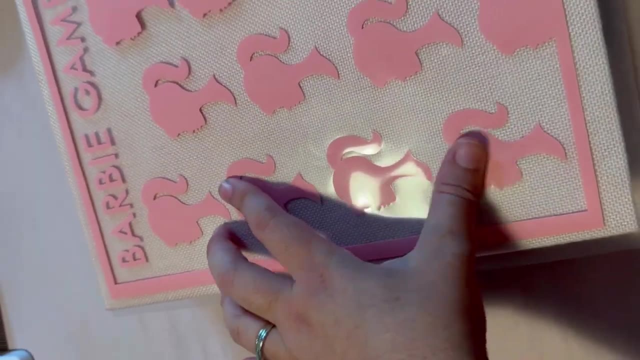 perfectly, because if you don't it's going to look crappy on the shelf and I did that so I know and it doesn't feel good. So the front was easy for me to line up. I'd put it there and stay there. The spine liked to move a little bit. I wish I would have got some heat resistant tape that I could. 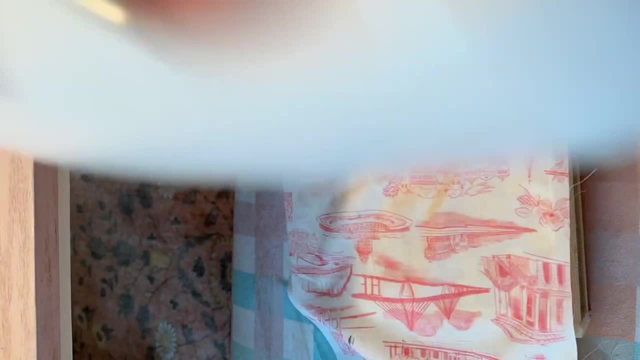 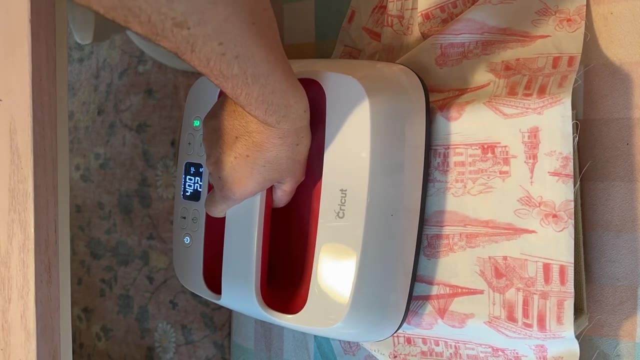 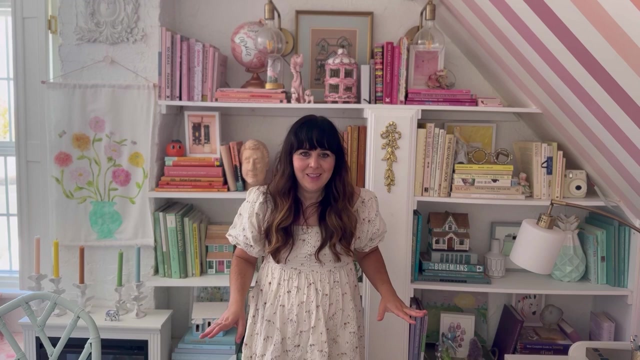 tape it on there, um, so that it would stay. So to adhere the iron-on onto those linen book boxes, I'm using my easy price. I set it to 400 degrees and I put it on each section for about 60 seconds and I push on it and then wait, wait, wait, wait, wait, 15 minutes. 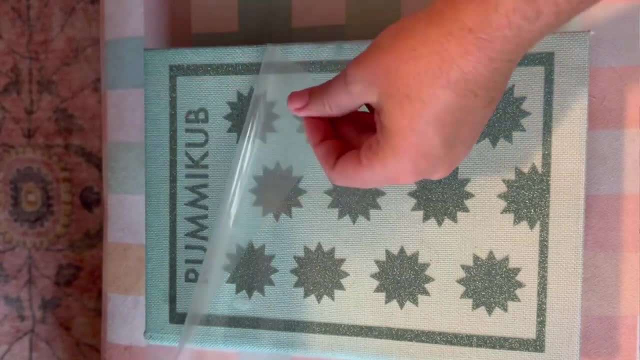 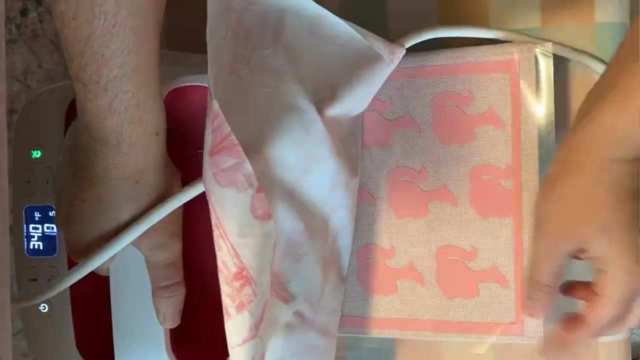 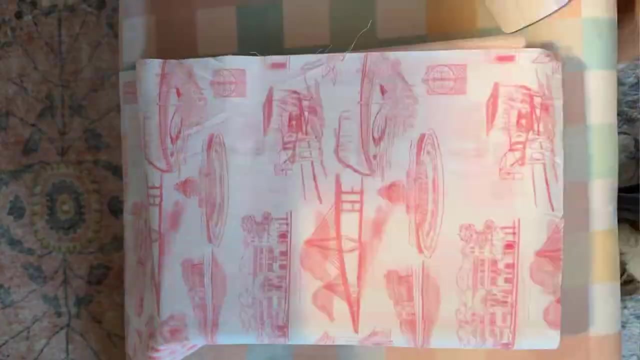 So it's totally cooled off and the plastic should come off so fast. I forgot about this. It's been a while since I've done this process, So I was like ironing and trying to pull it up and it was like bubbling up and it looked horrible. So don't do that. Press it for 60 seconds, Let it sit It'll. 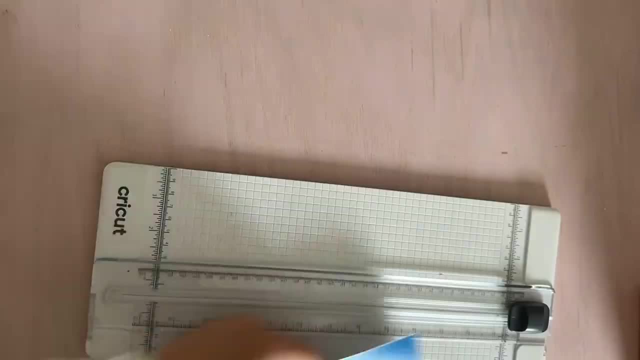 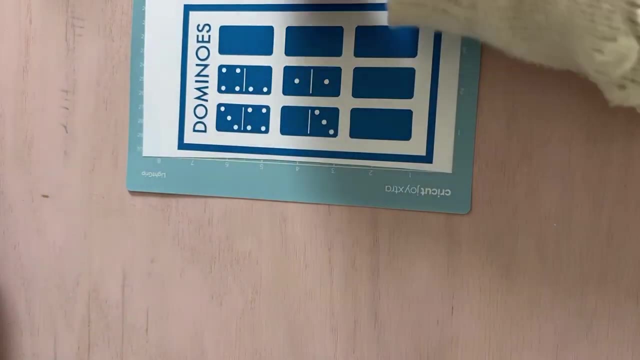 come off easy. So make your life easier and do that. So for the vinyl, the process is pretty much the exact same. You're going to weed it, Um, the one thing you need to do is you need to use transfer tape. So, once it's weeded, you're going to put it on the back of the book box and you're going to 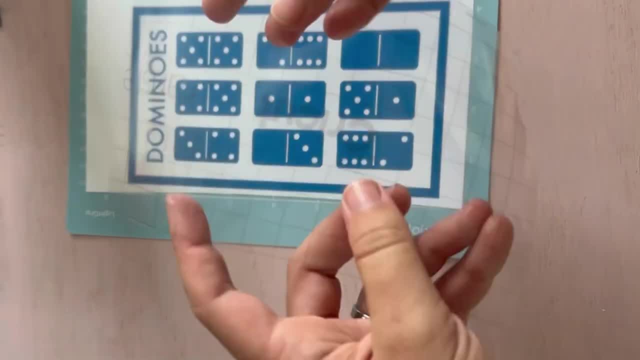 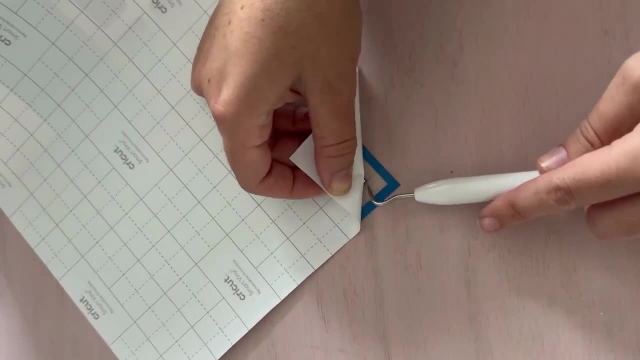 put transfer tape on the front of it and then you're going to pull the backing off and you have to be like slow and careful with this. And then you're going to put your transfer tape on top of the paper mache book and you're going to use something to like: push it down really hard. 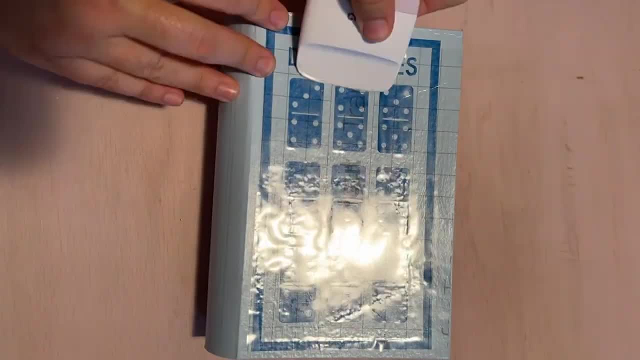 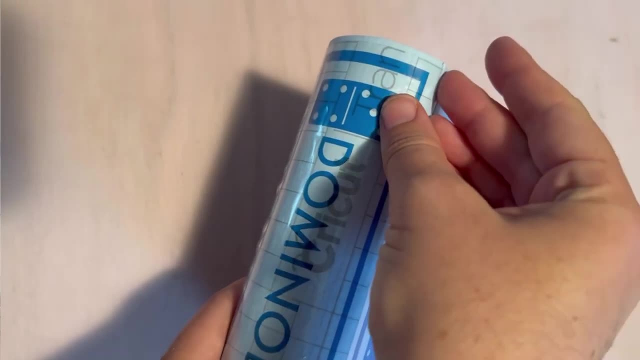 So you can use the tool that comes with Kricker. You can use like a credit card and then you can pull the plastic off and you'll have a really nice cover. I thought painting the paper mache was easier. The paper mache book was cheaper, but putting on the vinyl was trickier because you 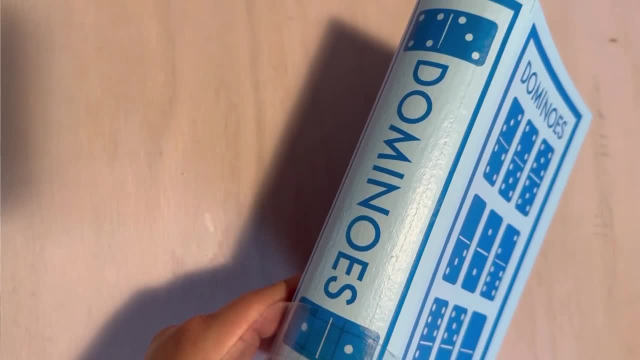 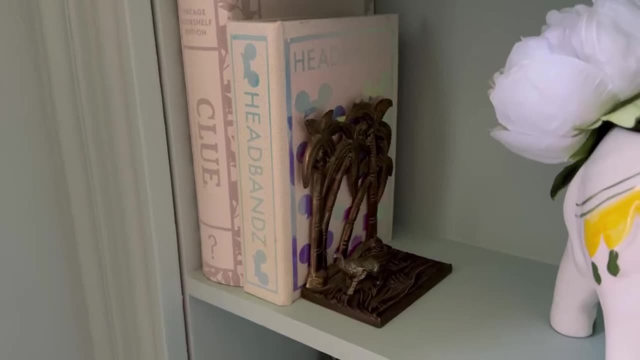 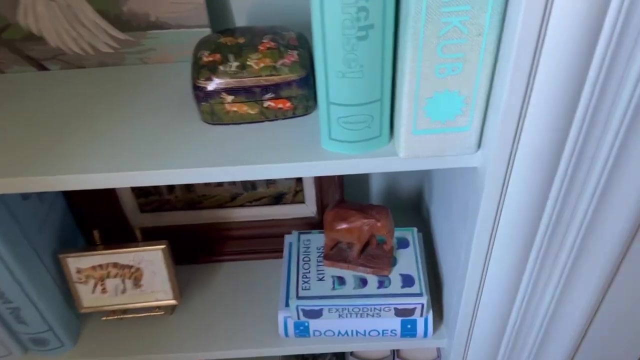 had to do the step with the transfer tape, and getting it right took me a while, Um, so it's just up to you which which you prefer. So it took me a full day, more than eight hours, to mix, to put the labels on seven boxes. So I'm not going to tell you that this is a very easy project, but it is. 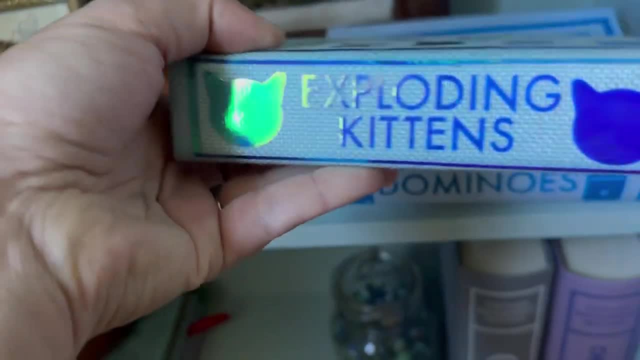 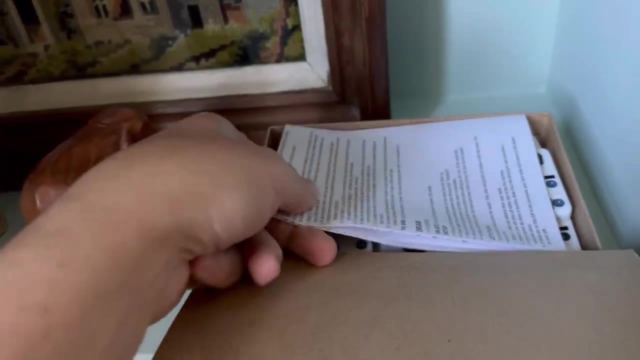 slow, and so I just like to be honest with how long it took me that long. but I'm a little bit rusty with Cricut, So if you've done Cricut recently, you could probably do it much faster than I could. I have all the labels done, You just put all the stuff in the boxes and it looks great. The only 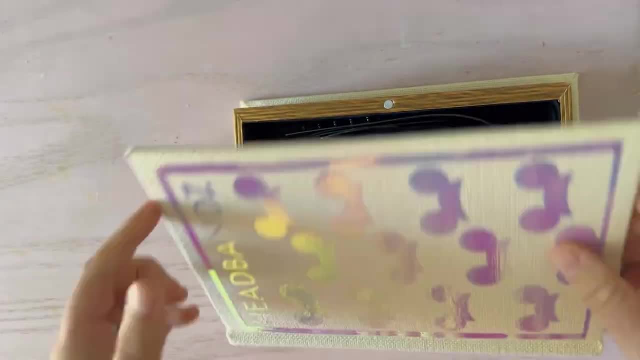 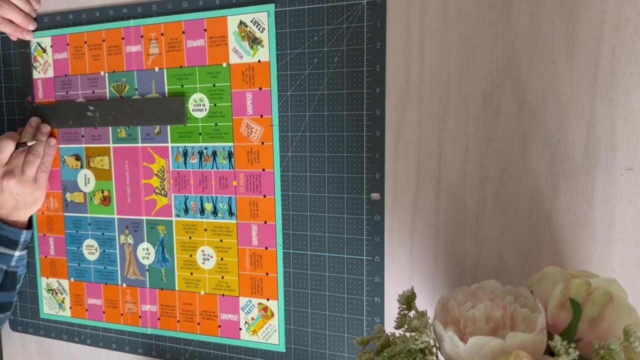 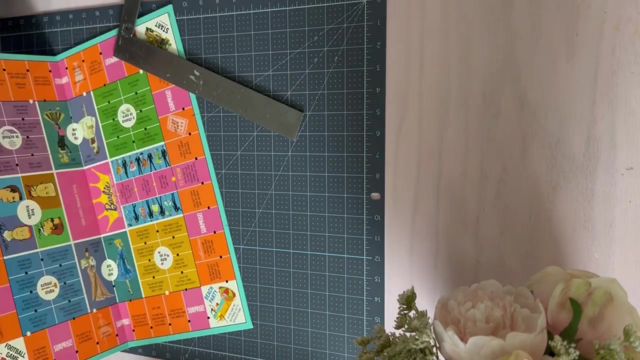 one I have a problem with is the Barbie game, and I love that game, but it's like long the board, So my husband cut it for me. I was kind of burnt out on this project at this point, so he cut it for me and we- um, I have the clue game from the vintage bookshelf game collection and so we just looked. at how that is. So it's cut for like two-thirds of it all the way through and then it's scored on other sides so you can be folded down into like sixths. and on one of them we cut it all the way and we just use book binding tape to fix it. but if you just score them, that's what we ended. 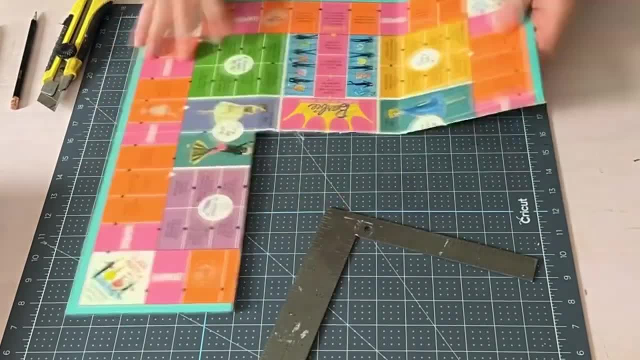 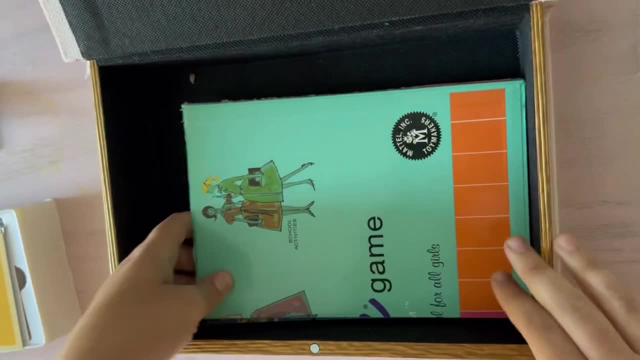 up doing on the rest, Like don't cut it all the way through just so the backing's still on there and it'll fold. It's way better. and when it's all open, even though it kind of looks dumb on the back, it still looks great on the front. So if you have some board games that you can cut down, this is a. 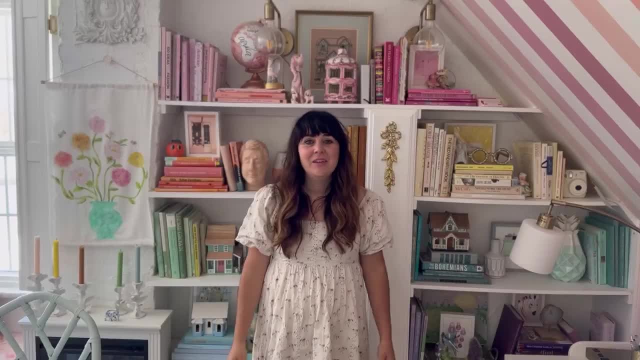 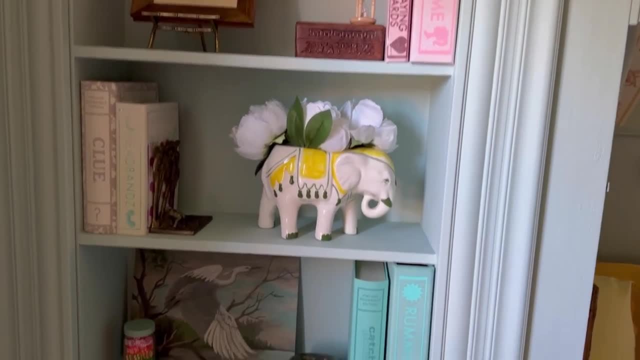 good hack. Okay, so that's this whole project. I wanted to show you how it looks like with all of them on the shelf. I think it looks so nice. It's so much better than all these misshaped board games, and I really love how the colors look on the shelf, and my son has been playing them more, so that works. 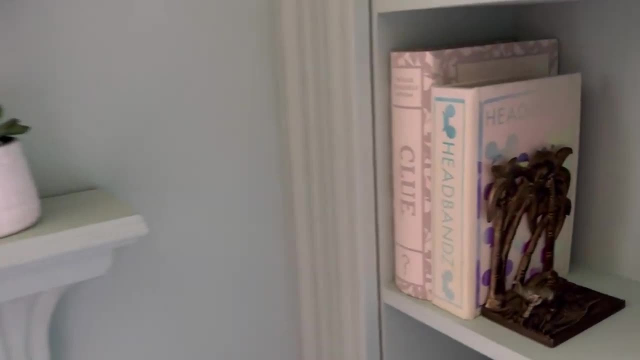 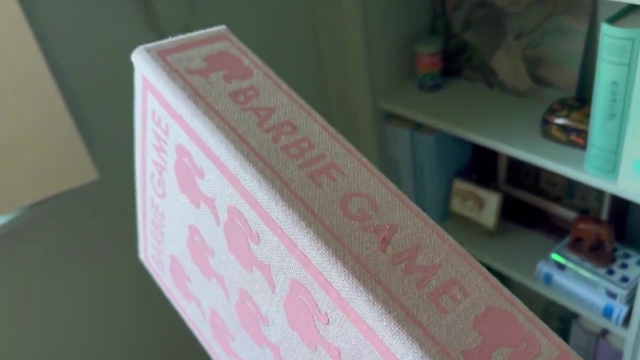 So I just think it looks so pretty to look at, and the holographic covers were definitely my favorite. I think they look amazing and they like turned out the best. so if you're gonna buy material for that, I'd probably suggest the holographic, because it's really cool. Um, and I matched the color of 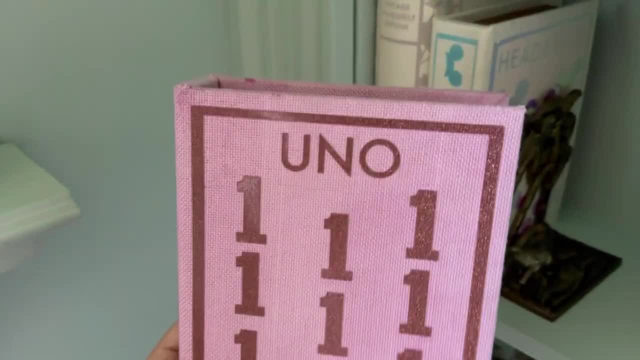 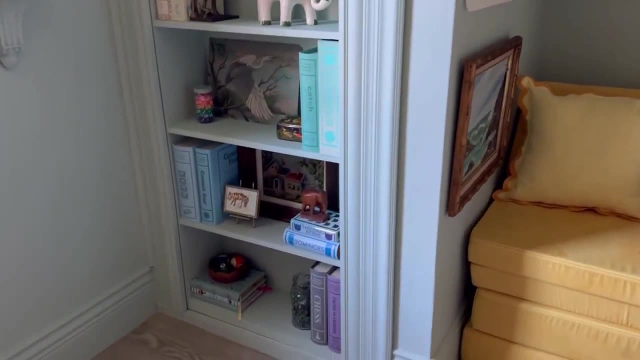 the vinyl to the color of the book box, because that's the color that I like the most. That's kind of how the other books did it and it turned out so nice. So, again, like I said, this is a really slow project, but if you want to like spend a weekend making something that, like you could have.